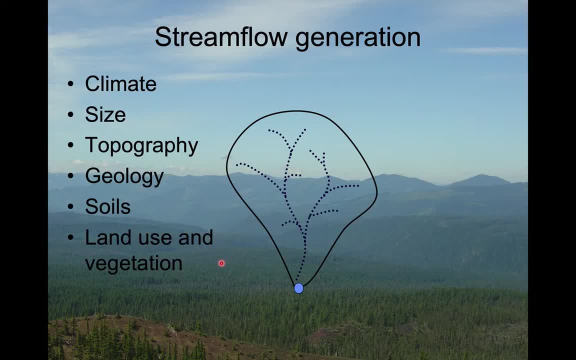 characteristics here. these are the ones we've been talking about all semester long, the sorts of things that we might be able to get from GIS data or stream stats or other things we know about the watershed and be able to understand how those characteristics influence the way water. 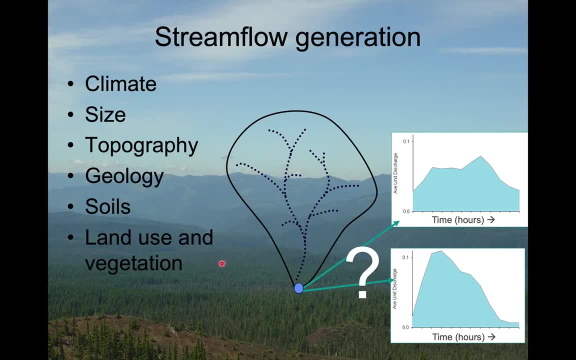 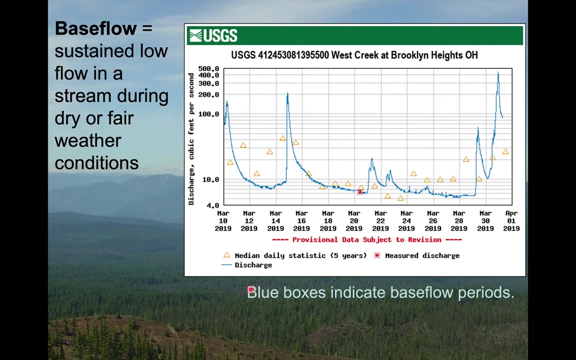 moves to the stream and ultimately do something like predict the hydrographs of the stream as a function of the watershed characteristics. Before we do that, we need to define some basic terms that you'll be hearing for the rest of the course. The first is base flow, So this is the low flow in a stream when it's not raining. 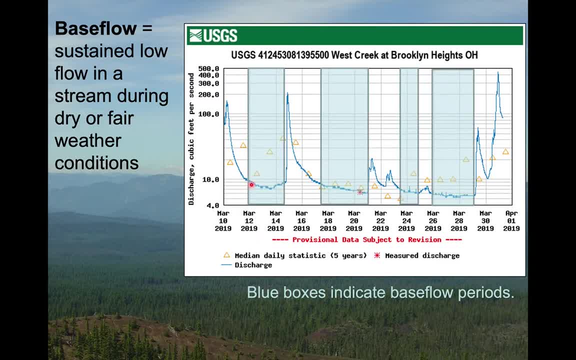 So I'm going to add some blue boxes to this example hydrograph here. So these blue box periods are the base flow periods, so times when it is not raining, when the stream isn't rising and when it isn't falling very quickly. In between, the blue boxes are: 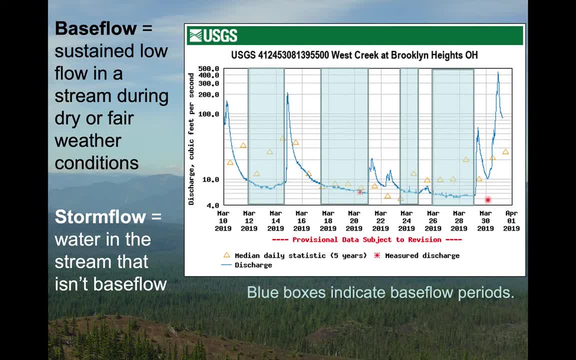 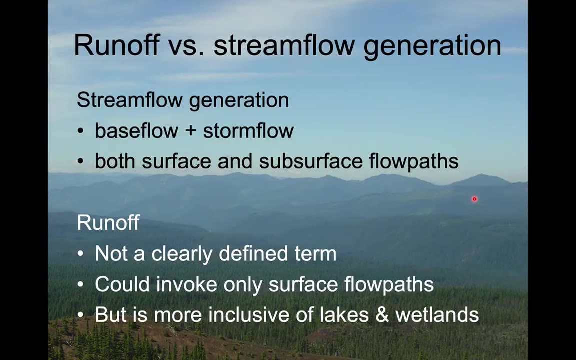 storm flow periods. So these are times when water is entering the stream as a result of precipitation that's occurring or that has recently occurred And, as a hint, we're going to have different stream flow generation mechanisms operating or different importance of them during storm flow periods versus base flow periods. Just a semantic note, a terminology note. I really 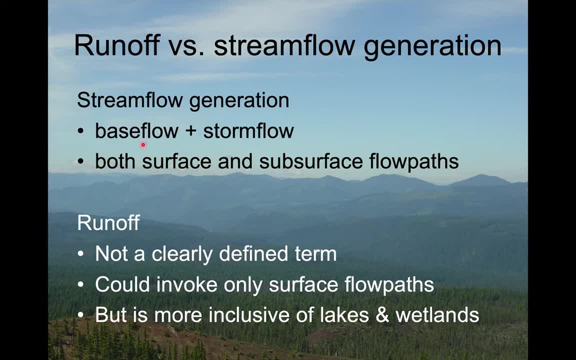 prefer the term stream flow generation because it incorporates both base flow and storm flow periods into it. So stream flow is base flow plus storm flow, And because we are thinking about both those base flow periods and storm flow periods, we are thinking about flow paths that occur both on 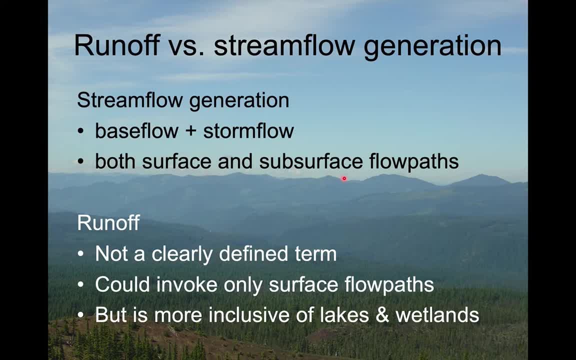 the land surface and those that occur in the subsurface. So that infiltration business that we've just been talking about, what happens to the water after that? You will see a lot in some of the resources that I'm linking and in some other videos, the term runoff generation mechanisms. I don't like this term quite as much because runoff 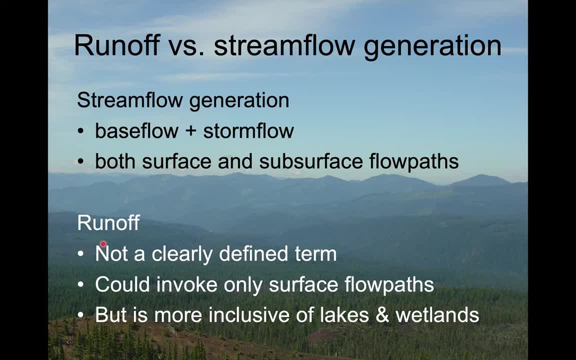 is not a clearly defined term And sometimes, when people are talking about runoff, they're only talking about flow paths that are happening on the surface. Well, so if we're only talking about surface flow, those are generation mechanisms that won't occur during base flow periods and will exclude some 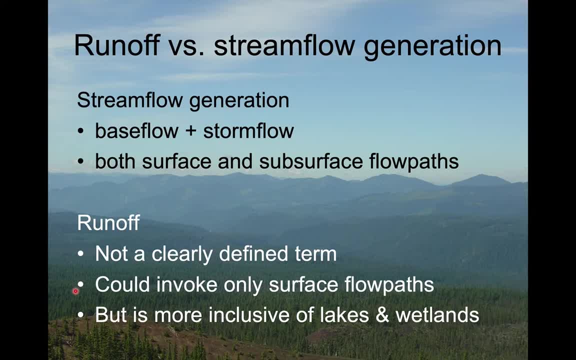 really important things. So it's not always clear to me what people are talking about when they say runoff generation mechanisms, which is why I use stream flow generation mechanisms instead. On the other hand, the word runoff and runoff generation mechanisms includes flow that gets. 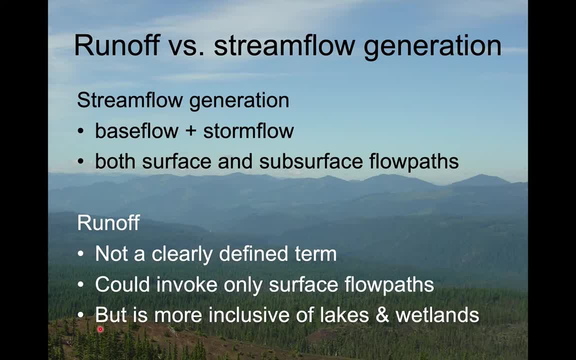 to lakes and wetlands instead of streams, or before it gets to streams. So I prefer the term stream flow generation mechanisms ignores that. So six of one, half dozen of the other, But just know that more or less stream flow generation mechanisms and runoff generation mechanisms are. 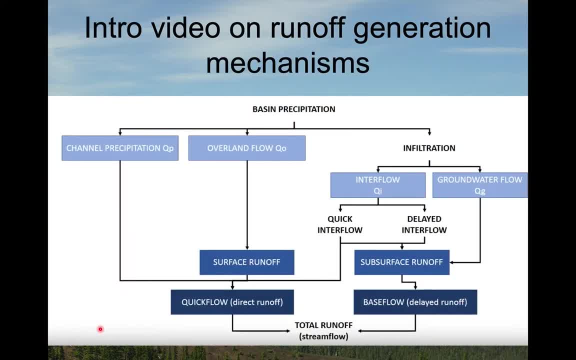 really referring to the same set of processes. Just below this video you will find another video that really kind of breaks down all of the different ways that water can get to streams, these runoff generation or stream flow generation mechanisms. So Encourage you to watch that first below. 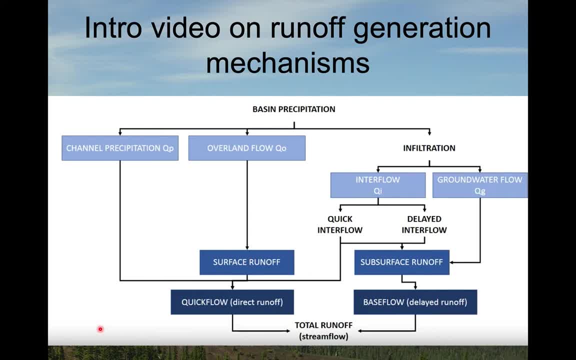 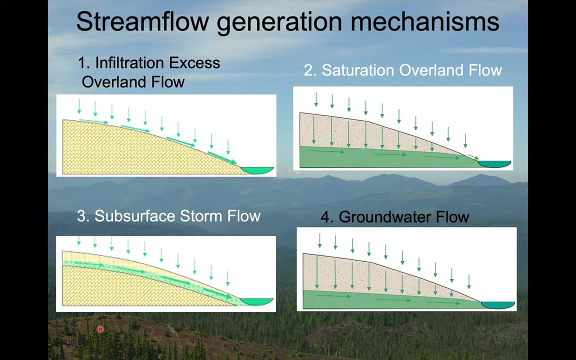 That is a link to a web page, or rather a whole series of web pages, that take you through these flow generation mechanisms and the watershed characteristics that control them. So that's sort of a good supplement to your text for this session of the course. And then what you'll see in that video and in that web page is there really four important processes to move water. 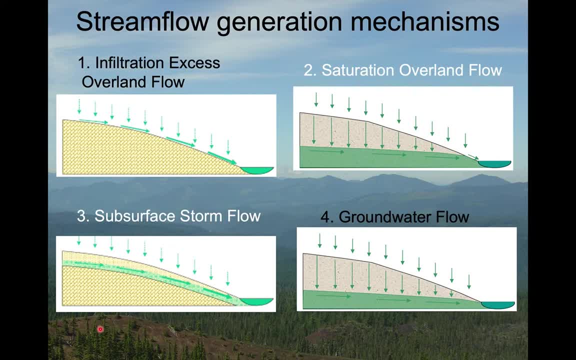 from the watershed into the stream: infiltration, excess overland flow, saturation, overland flow, subsurface, storm flow and groundwater flow. So I'm going to make a series of short videos that will take you through each of those processes or link you to some other. 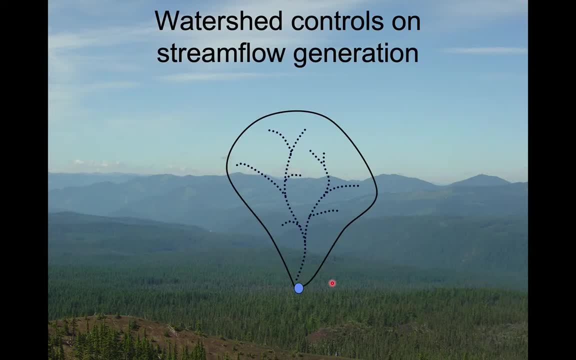 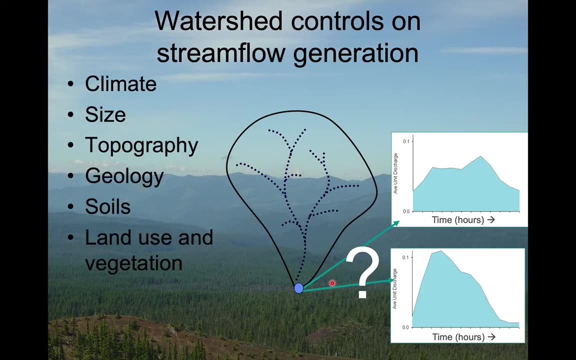 resources for each of those processes So that ultimately, again, the goal is that we know something about the watershed and are able to predict stream flow from the landscape characteristics. But I'll tell you the short answer right now. it's complicated, so we're never going to be able to have a one for one. 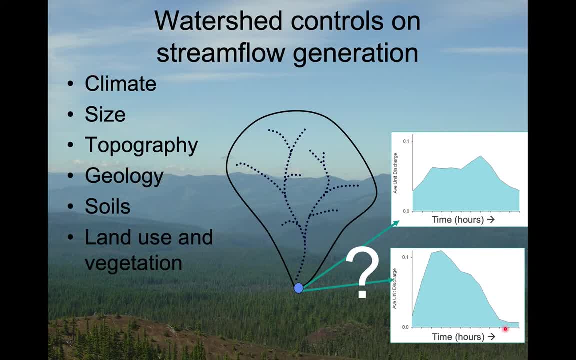 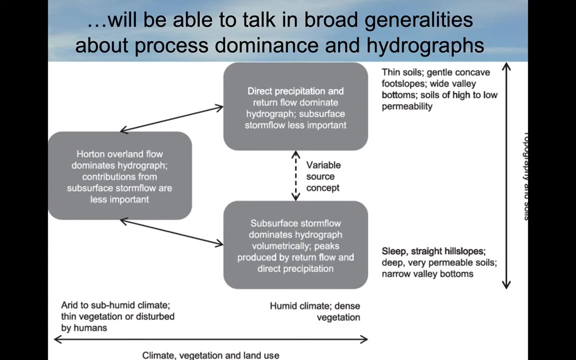 relationship between things you can read off a map and knowing exactly how a stream will respond. You need some pretty complex hydrologic models to be able to do even a reasonably good job of simulating stream flow from watershed characteristics. Instead, where we'll get to in this class is to be able to talk.